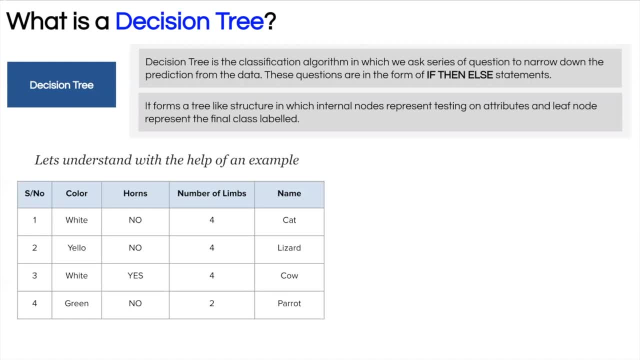 if you are not able to get this, let us understand this with the help of an example. This is a table which represents the characteristics or attributes of animal, like color, number of limbs, whether animal has horns or not. Based on this, we will be able to determine: 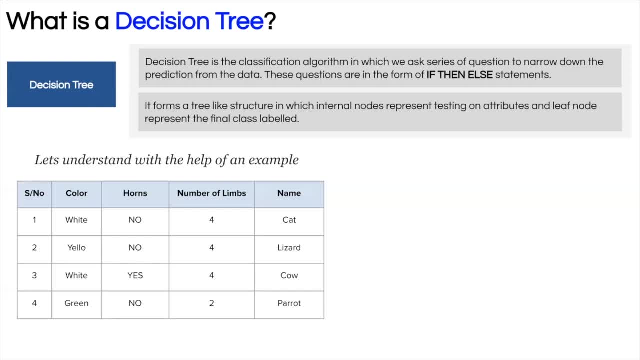 the classification model. So let us assume we want to create a classification model which can classify animal into cat, lizard, cow, parrots, depending on the attributes. So how will we go about it? We will ask a question whether the animal has horns or not, If it. 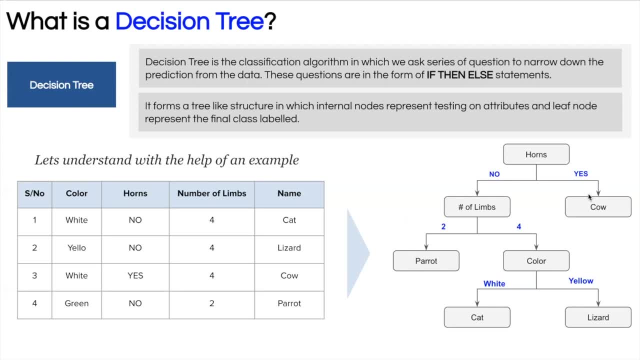 has horns, then it will be a cow, because from the data and from the table we can see that only one animal has horns. Then if animal doesn't has horns, then we go on asking: what are the number of limbs animal has? So if it is 2, then it will be a parrot. If the 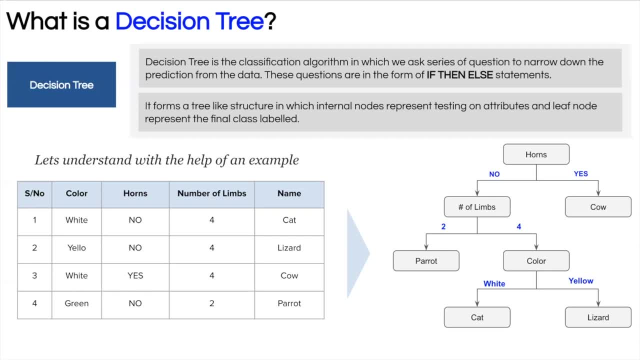 number of limbs are 4, then we will go on and asking one more question, depending upon their color. So that is how we create a decision tree, And these are the leaf nodes. These are the leaf nodes which actually tell what the final prediction is. So this is how the 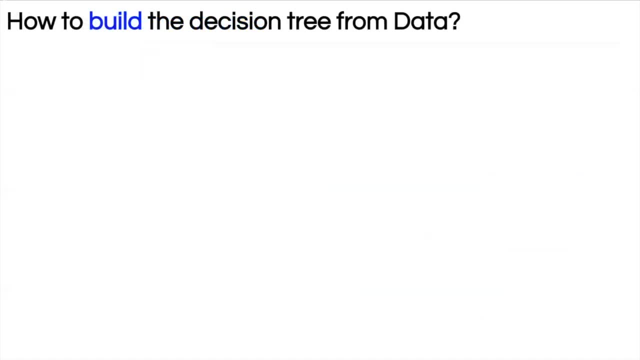 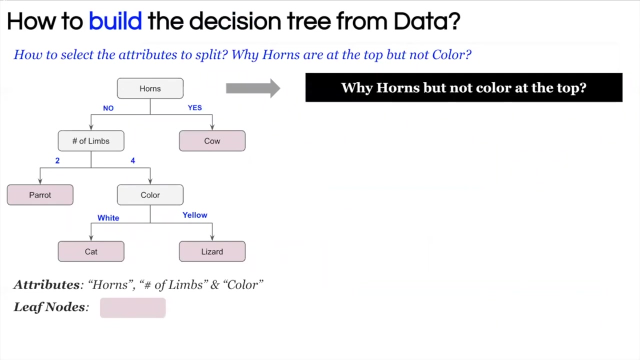 decision tree looks like Now. the next question you would have in mind is: how did we build this tree? Why did we ask the question related to the horns but not the color or other attribute? Why not number of limbs? Why horns but not color at the top? So this is the basic question. 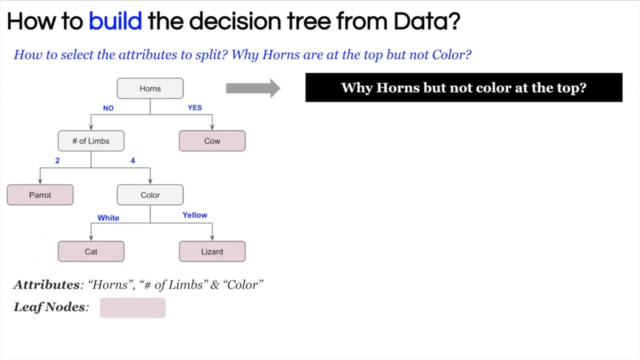 which you will have in mind. So what we do is like we use an objective function. The goal of this is to get the most efficient tree, So we choose the attribute in such an order that decision tree can cover the entire data in minimum number of attributes. 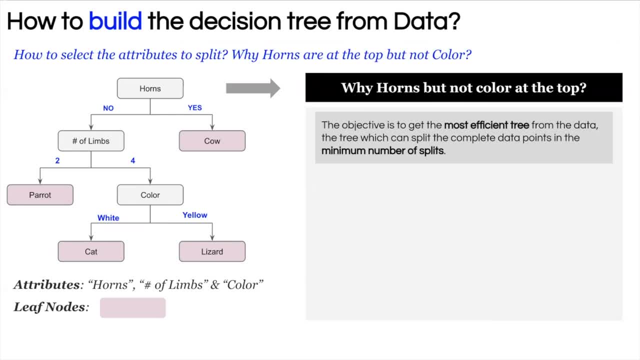 So what we do is like we use an objective function, that is, information gain. Maximization of this objective function is tied to our goal of the efficient tree. So if you maximize this objective function, our goal of the efficient tree will automatically reach Next question. 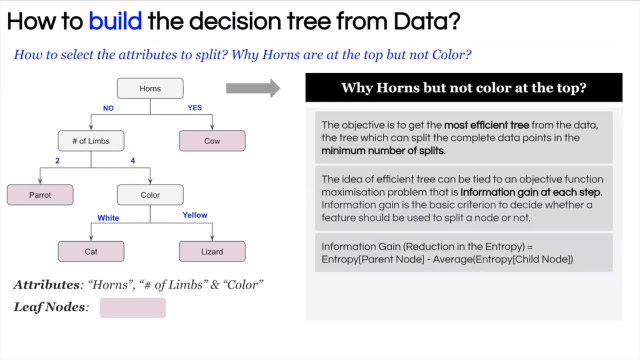 is: how does this objective function looks like? So the objective function is defined as the entropy of the parent node minus the average entropy of the child nodes. So at each step we can define the entropy of the parent node minus the average entropy of the child nodes. 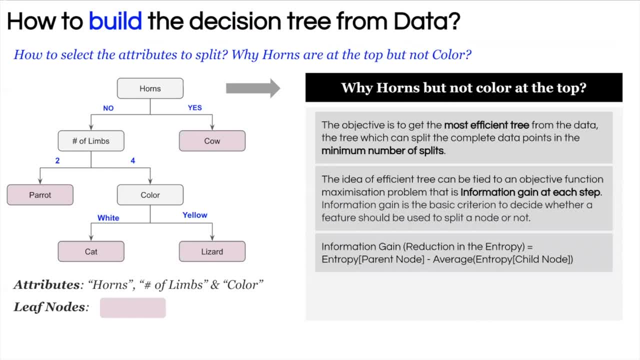 So we calculate the objective function using different split and see which split is maximizing it and use that splitting attribute. So what we do is like: while creating this decision tree, at the very first step we use different attributes like horns, number of limbs and 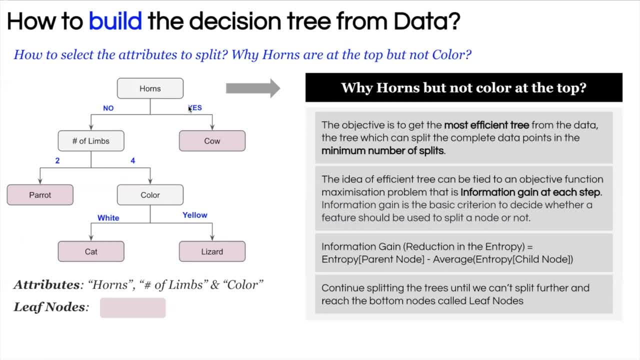 color and create the first step of the tree. Then we calculate this objective function of the information gain. So how we do is like we calculate the average entropy of horns and we subtract the average entropy of these child nodes and we do this for all the attributes, like horns, number of limbs and color, and see which attribute. 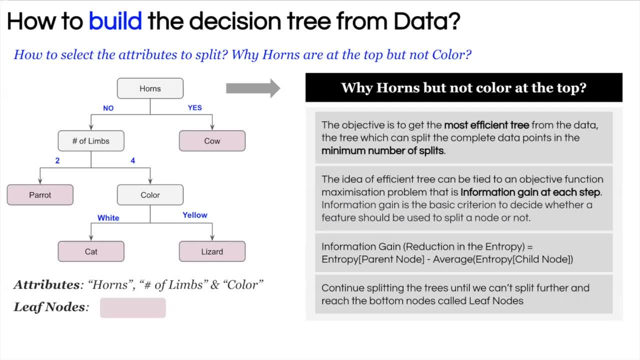 is giving the maximum information gain. So in this case, the horns might be giving the maximum information gain. that that's why we choose it at the very first. Likewise, at every step, we use this and get the complete tree built. Now, once we have that, we can. 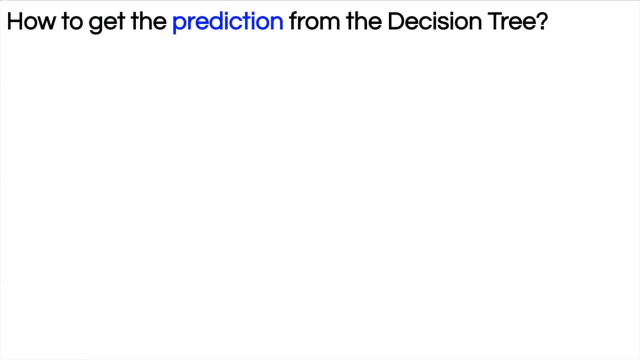 see that the data. we have designed the decision tree. Now how do we use this tree? How do we get the prediction? So there can be two different type of tree, like decision trees and regression tree. Decision trees we have already seen in the animal example, because 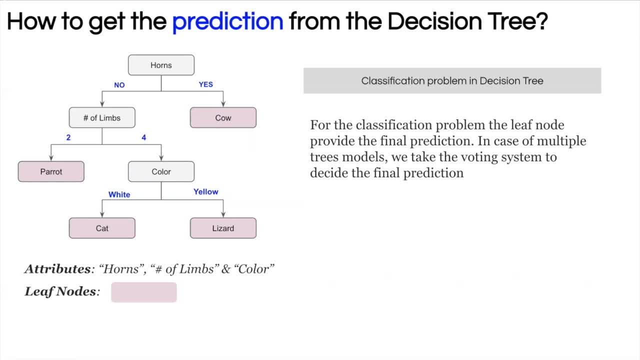 they are. the classification output was categorical and in case the regression tree, the classification is the numerical variable. In both the cases the output is decided by the leaf node. So if you want to do prediction on the leaf node, you can use the leaf node. So if you want, to do prediction on the leaf node, you can use the leaf node. So if you want to do prediction on the leaf node, you can use the leaf node. So if you want to do prediction on the leaf node, you can choose the leaf node, But in case, if you want to do prediction on the leaf, 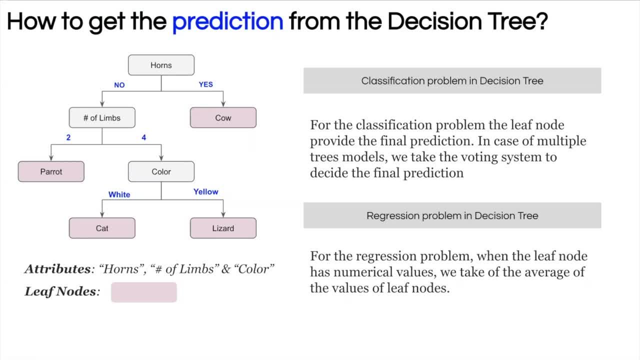 node. you can choose the leaf node. So in the case of the new data, what you do is you map it to the tree and see where it is falling in the tree. Which leaf node does it fall in? That is your predicted class. In case of the regression tree, we might have to do 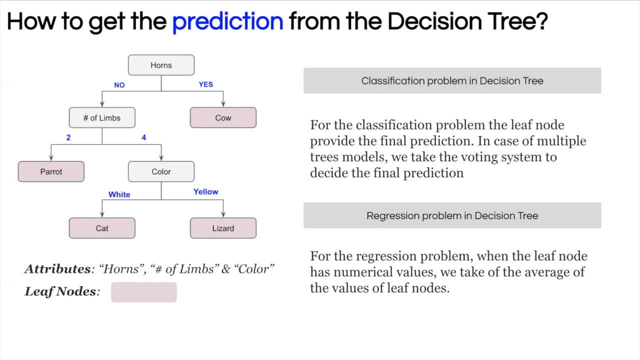 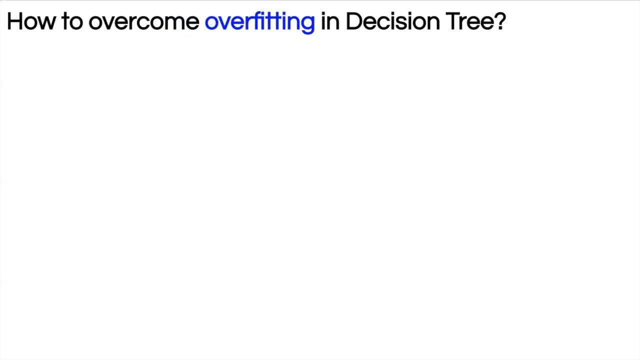 some kind of computation in terms of average, median mean, etc. to get the final prediction. Till now we have understood what are decision trees, how to build decision trees and get the prediction. But now we will see how to overcome the problem of overfitting in. 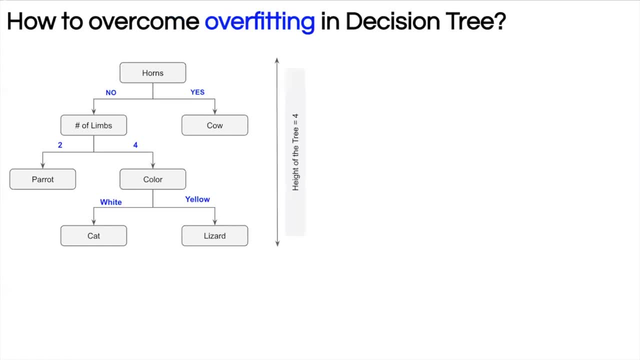 in the decision trees. This is one of the very common problem which we face while building decision trees as well. like any other machine learning problem, The problem of overfitting and underfitting is closely tied up to the height of the tree. If the height of the tree is too much, 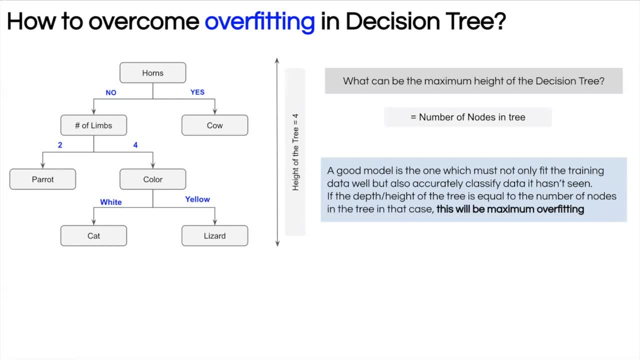 then it will cause overfitting and shallow tree will cause the problem of underfitting. Please think about it very carefully and let me know the reasoning in the comment section. If you want me to explain this point in great detail, I'll explain then, and there only So, the 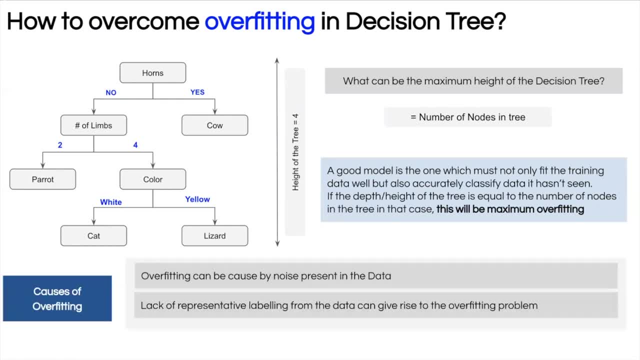 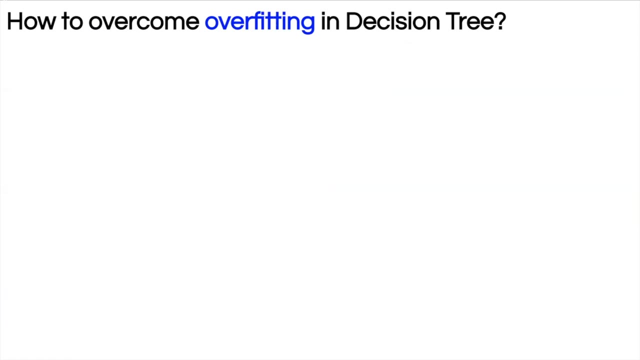 problem of the overfitting in the decision tree can be caused by various reasons. One can be noise in the data. second can be lack of representative labeling from the data. These are two primary source of the overfitting in the decision trees. Now let's see how to overcome the overfitting in. 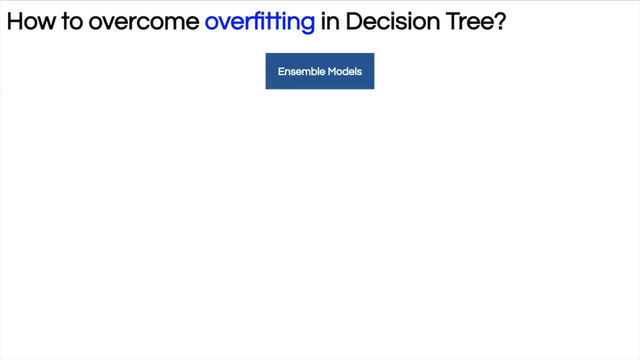 the decision tree. So the popular strategy of overcome the problem of overfitting is the NCE. The goal of ensembling is to combine multiple models, to create a meta model which can better generalize the result on the new data. How can we combine multiple models? 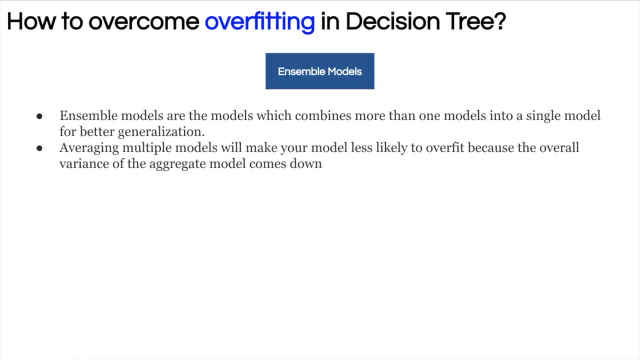 There can be various aggregate function like average, median or maybe some of the complex functions. So how do we create ensemble model for decision trees? So it started with splitting your data into multiple data sets, Then get the decision tree classification for each of the data sets. So you can get the decision tree classification for each of the data sets. 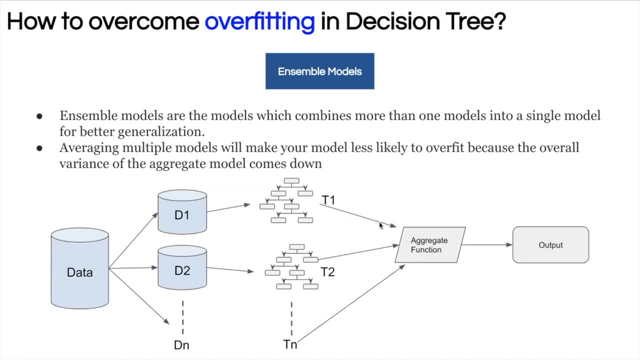 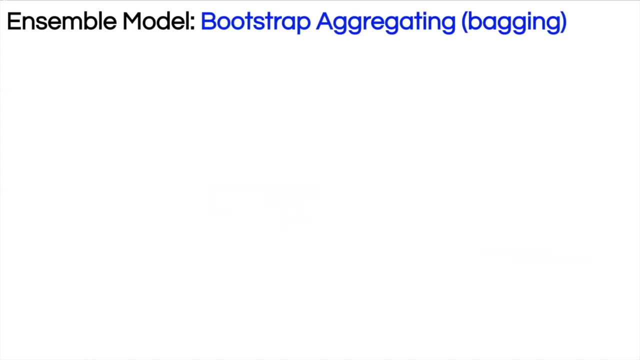 Then we generate the prediction from each of these decision trees, then combine them using some aggregate function like weighted average, median mode, etc. to get the final prediction. This is how the ensemble model works. So one of the most common method to build ensemble models is bagging. 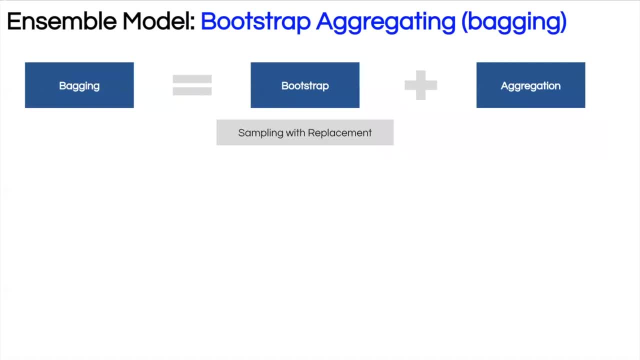 which is actually bootstrap plus aggregation. So bootstrap is basically getting the data sample with replacement. This process is known as sampling with replacement. You might have already studied in plus 2 or in undergrad. So what we do is like we get the samples from the data to train the model and replace it back So we can get the same observation. 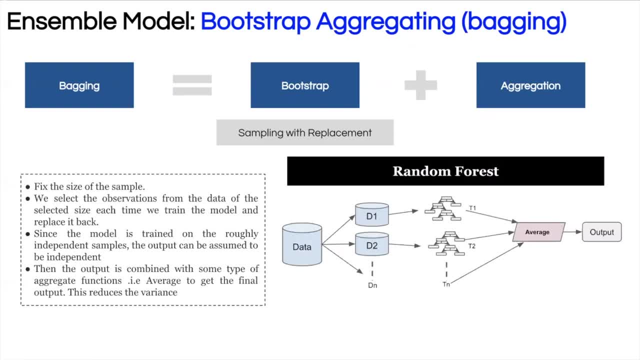 in the sample because we continue to replace it back. Random forest is a type of bagging model where the aggregate function, where the aggregate function is the average function. So what are the steps? The steps of getting the random forest is is stated here. So what we do is like we fix the sample size, Then we select the observation from. 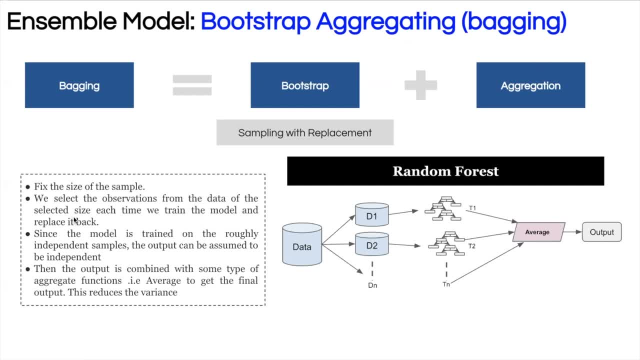 the data of the selected size each time we train the model and replace it back. That is sampling with replacement. Since the model is trained on the roughly independent sample, the output can be assumed to be independent. That is by the variance reduce and the problem of overfitting. 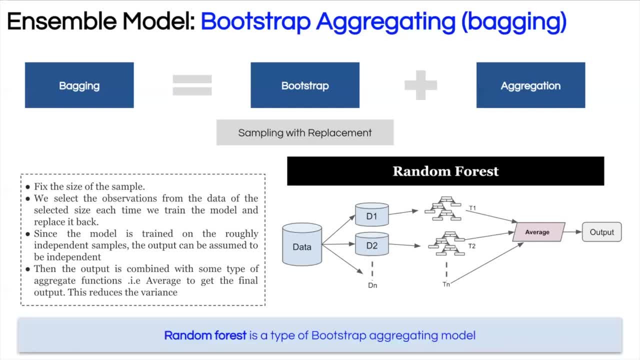 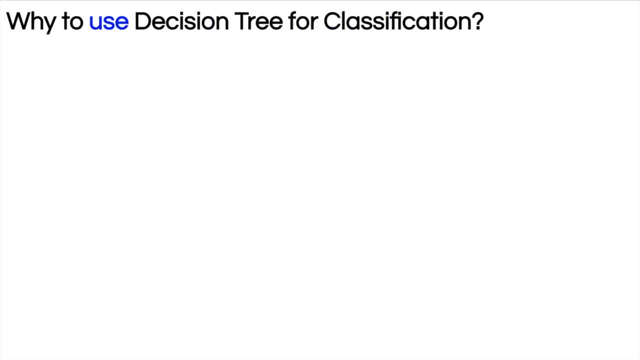 also reduces. So, all in all, random forest is a type of bootstrap aggregating model. So the last we can discuss about why to use decision trees in the classification problem. There are several advantages of using decision tree for classification problem, As algorithms have their own shortcomings as well. 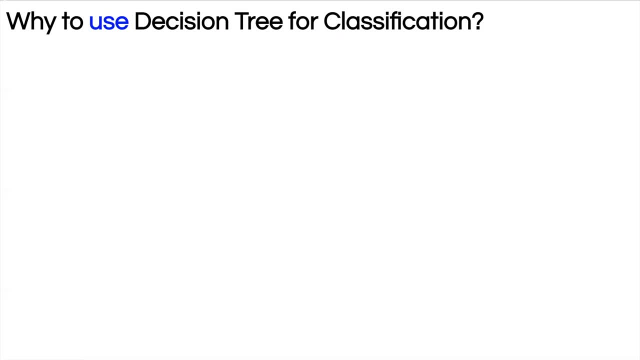 Likewise, there are disadvantages of using decision trees also. So let's first discuss about the advantages of the decision tree. So like you have already seen how easy it is to comprehend the decision tree, There are very interpretive also. these are PN Pandas over there also. So that is again. so because you listen in towards the algorithm and you lead by yourVA And then, if you have- so that means personally- you will fold and maybe document your argument. So there are some officers using decision trees as well, However, as�adi and meets the 수가 organs for helping you. 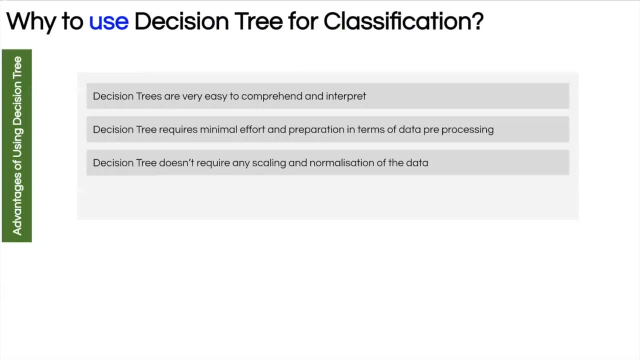 now. So let me conclude alone. this is the fact, as we are considering this topic as well, Where this theme of discussing Also decision trees don't require much of effort in terms of data processing. These pre-processing can be of different type, including data normalization, scaling of the. 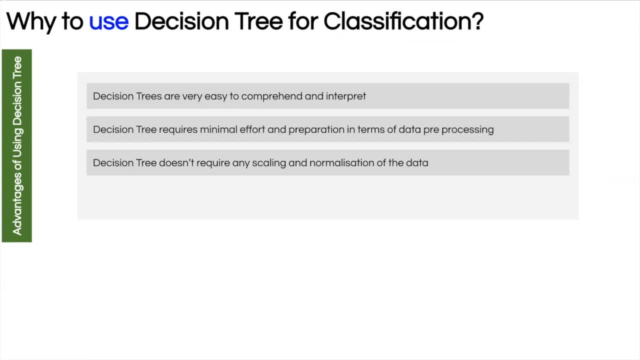 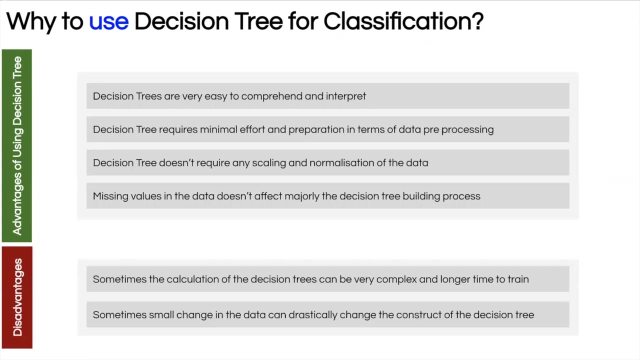 data and missing values also don't adversely affect the decision tree building process. These are the reason why decision trees are used for classification problem. There are some disadvantages as well. Sometimes the calculation of the decision tree can be very complex and time consuming. Also, the small changes in the data can drastically changes the structure of the tree. 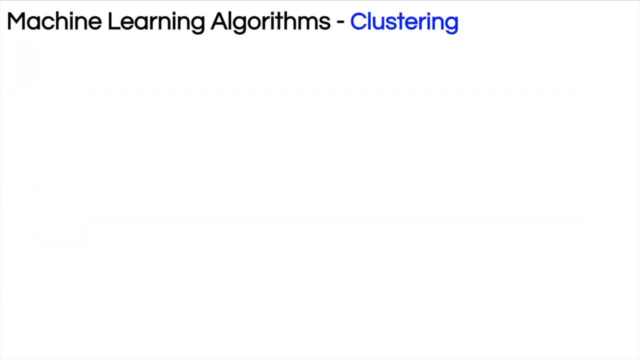 These are some of the disadvantages. With this, we have come to the end of the decision tree. By this you have conceptual understanding of why, what is decision tree and how do we use them. In the next module we will discuss about one more machine learning algorithm, that is, cluster.